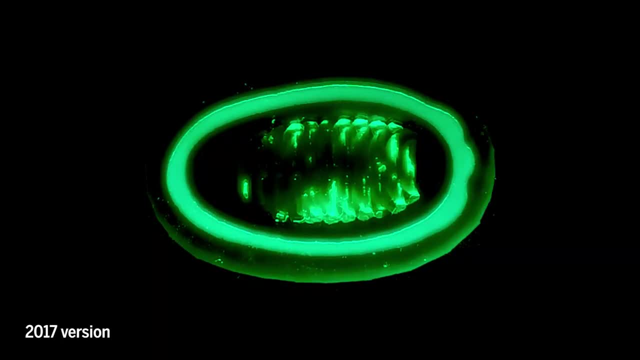 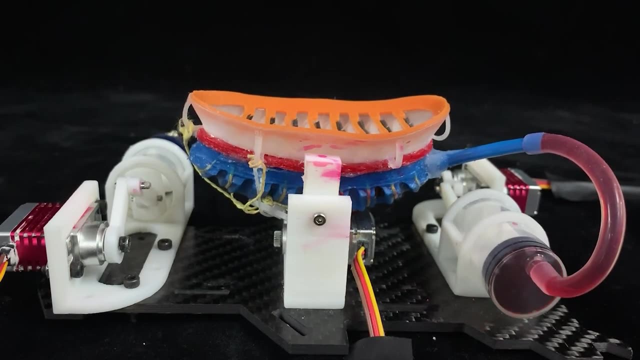 Getting rid of the tether and making the disk suction not just with the outer lip but also adding space. The researchers installed two very small water pumps on the robot. One pump bends the disk to position it along a surface, while the other controls the lamellae. 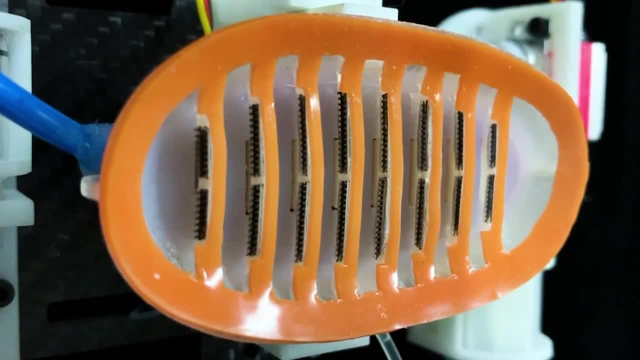 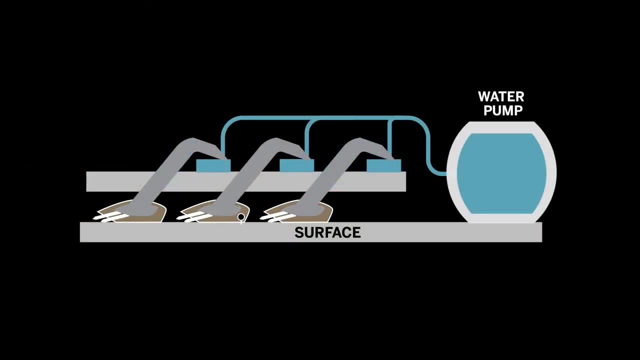 Once the disk presses down on a surface, a tight seal is created. from the difference in pressure between the compartments and environment, as well as the slight rotation of the lamellae To make the robot latch even stronger, fluid is stored in the robot's body. 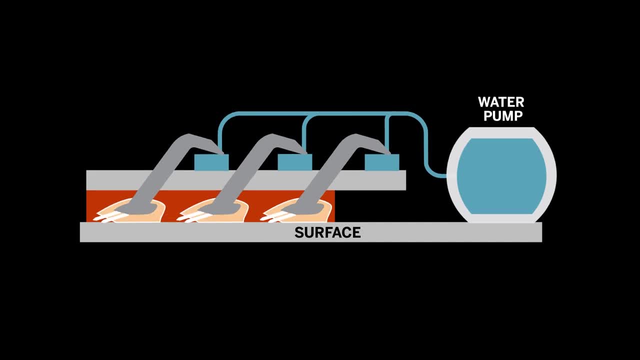 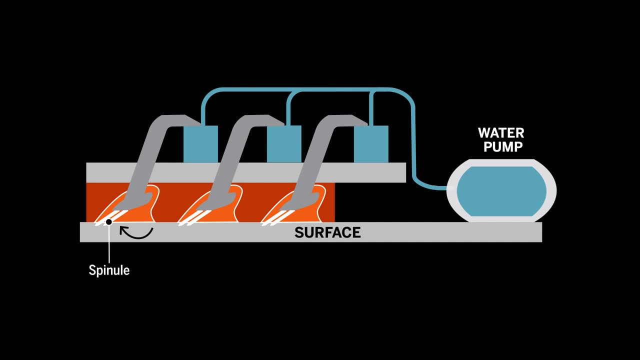 and the robot is able to move. To make the robot even stronger, fluid is pumped from the chamber back to the lamellae. This further rotates the lamellae and engages the spinules. It also reduces the pressure in the compartment, improving adhesion even more. 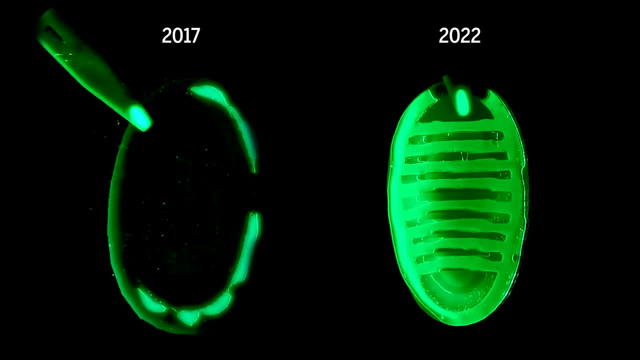 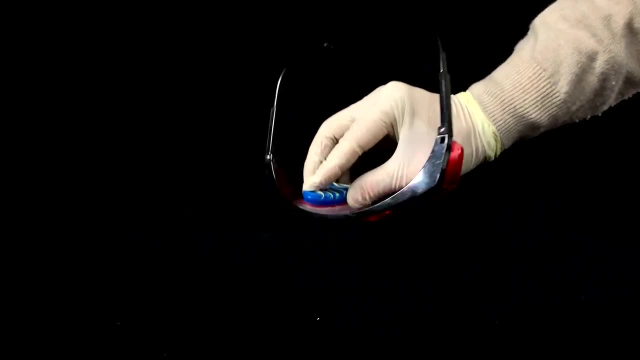 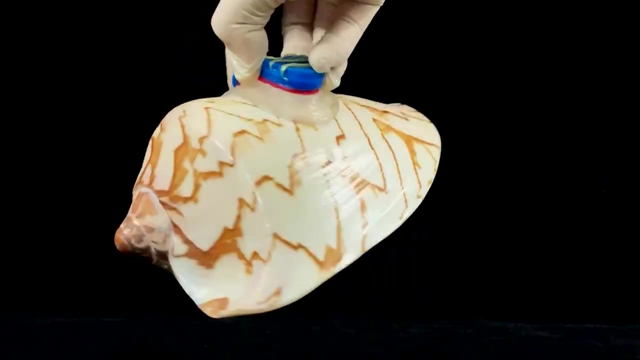 By creating multiple seals, the disk can stick around, even if some of the compartments aren't firmly attached. just as the researchers observed in real-life remoras, The disk could latch on to a variety of surfaces, both in the air and underwater, from the curved, smooth shell of a mollusk. 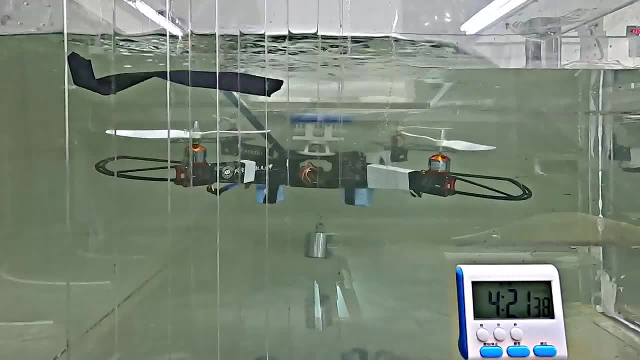 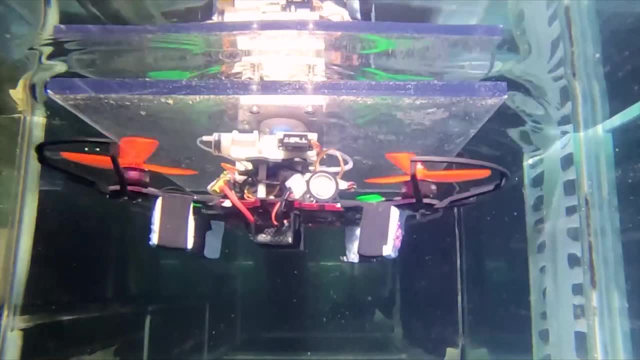 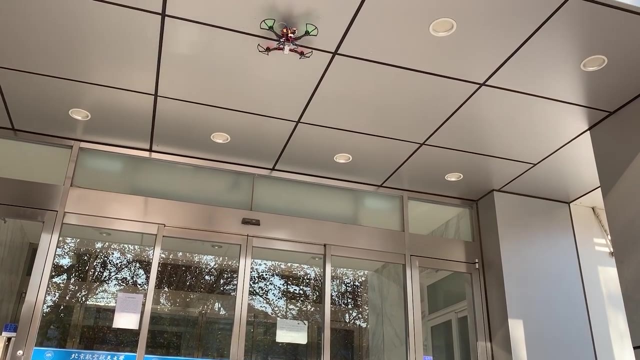 to surfaces riddled with microorganisms. The disk can stay attached to surfaces for hours and even hitch a ride onto moving objects. Next, the researchers channeled the capabilities of a kingfisher and added flight to their hitchhiking robot. The robot uses propellers to swim to the surface. 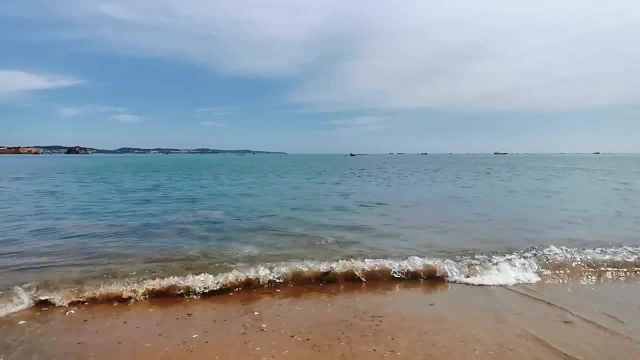 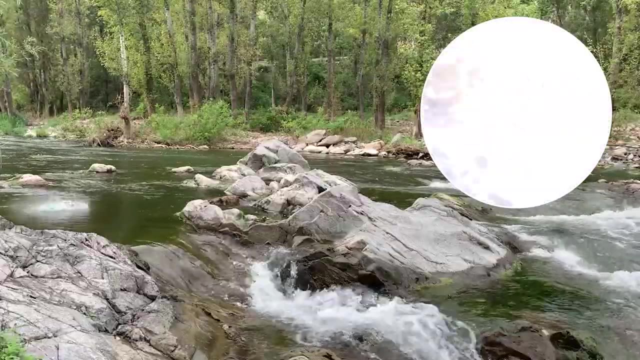 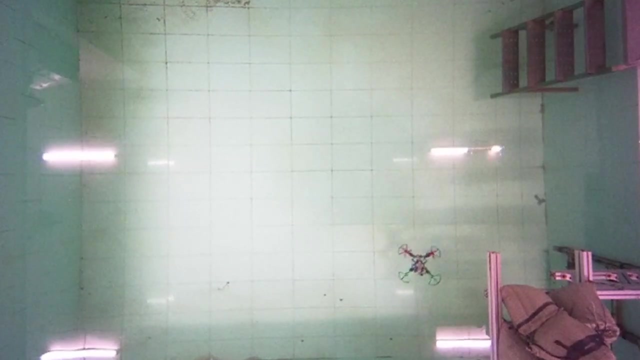 then shoot itself out of the water In less than half a second. Outside the lab, the robot proved it could deal with different environments. Throughout these excursions, a camera on board provided a view of the surrounding environment. While the robot can only swim up to a depth of about two meters, 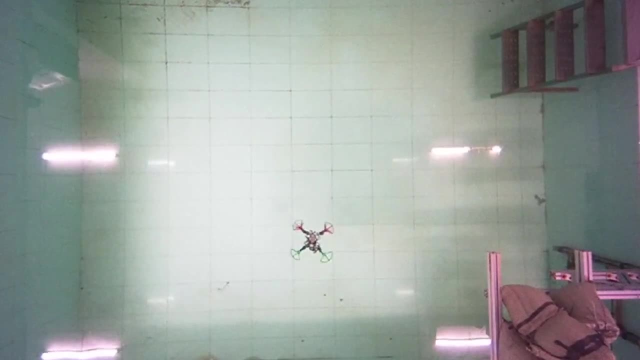 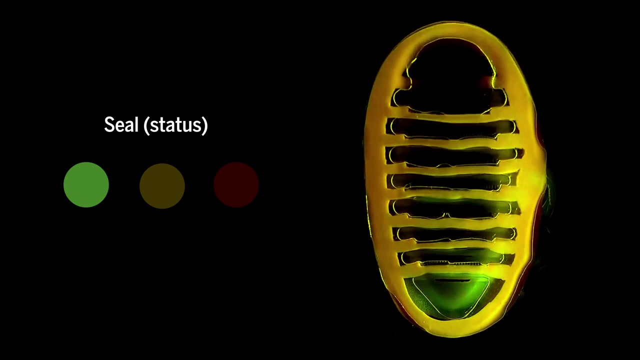 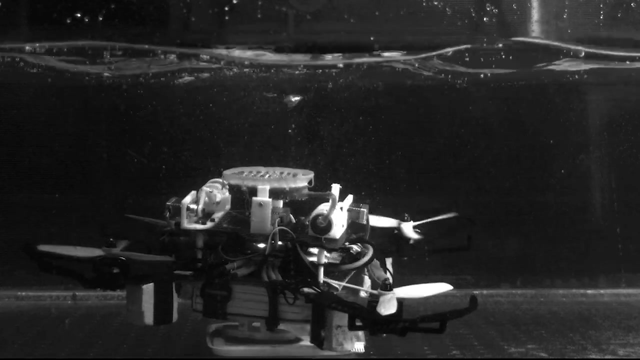 before wireless communication cuts out, it can continue to record at greater depths In the future. the researchers hope to add other monitors on board, such as a sensor to detect when the disk is fully attached or if there's a leak. Someday this little bot might be diving for your phone. 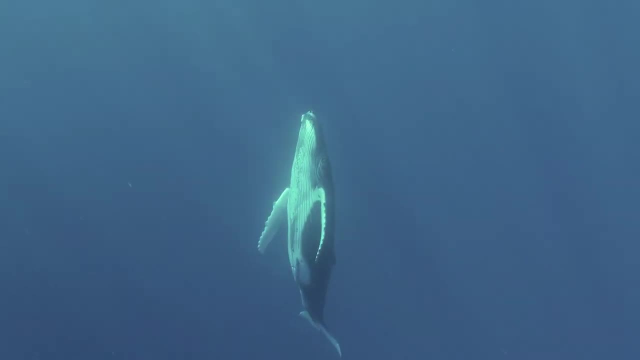 when you drop it off the boardwalk or riding along on a whale's journey.